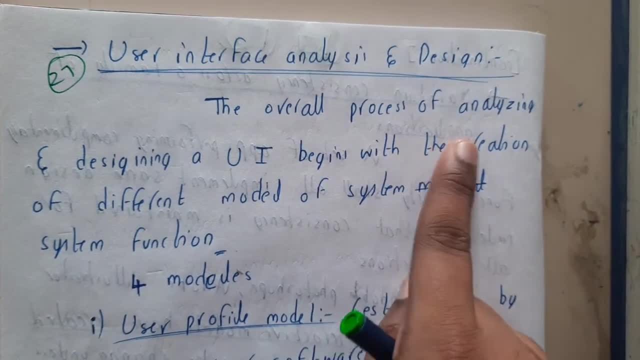 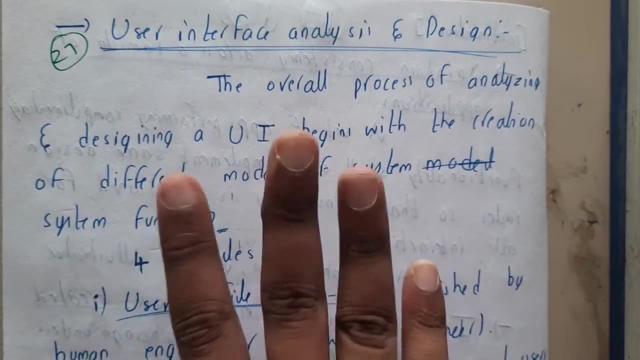 we will be going through analysis models and everything. okay, So the overall process of analysis and design of a UI begins with creating of different models, guys, okay, So here we will be learning about four different models. okay, So the first model is user profile model. 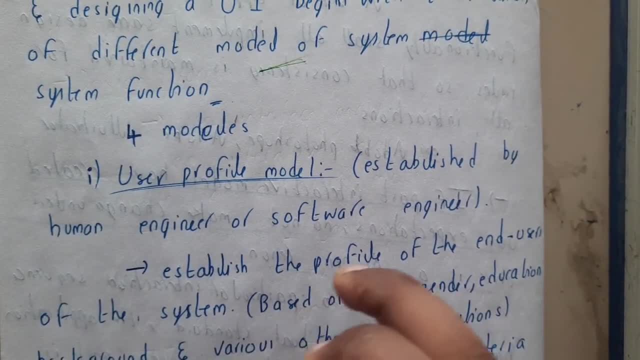 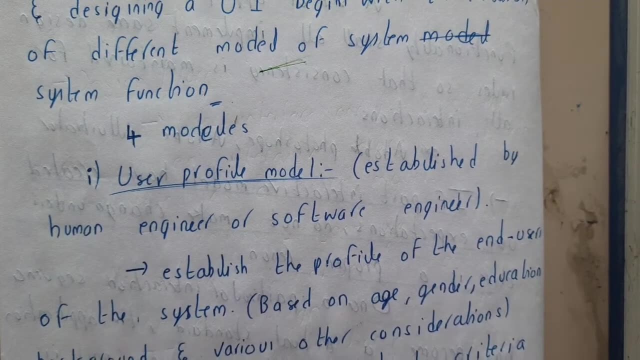 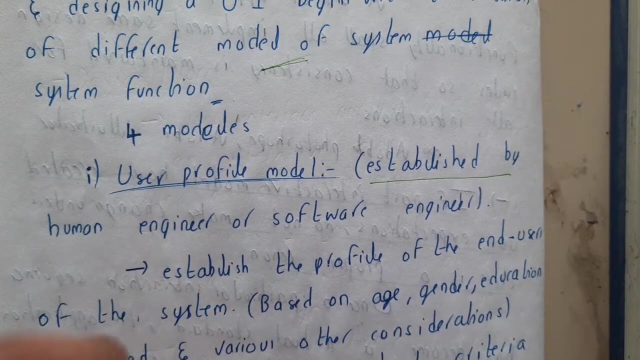 okay. So basically, this model helps in establishing the developer, how, sorry, how the interface should be or how the user will interact with the system. okay, It establishes it is established by- by a human, human or a software engineer. okay, Establishing the profile of the end user, of the 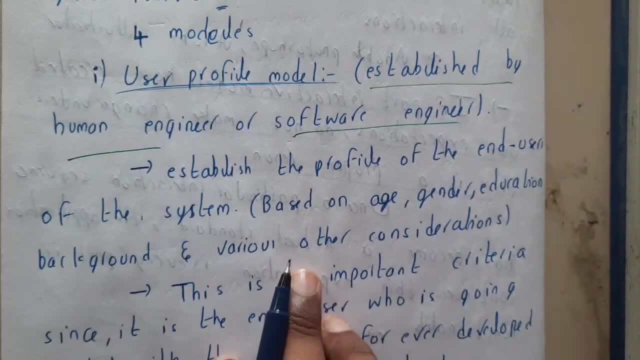 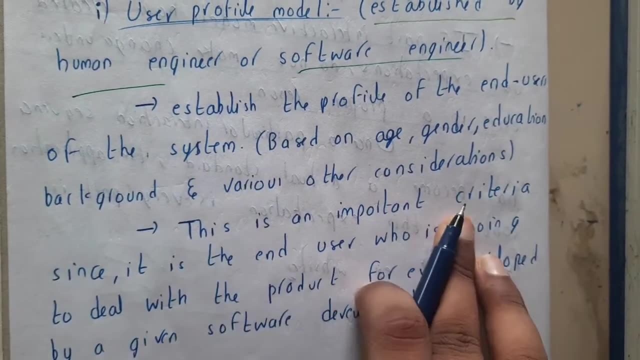 system based on his age, gender, education, background and various constraints. So you will be collecting all those constraints and you will be analyzing his view or how he is interacting with it. So this is an important criteria, since it is the end user who is going. 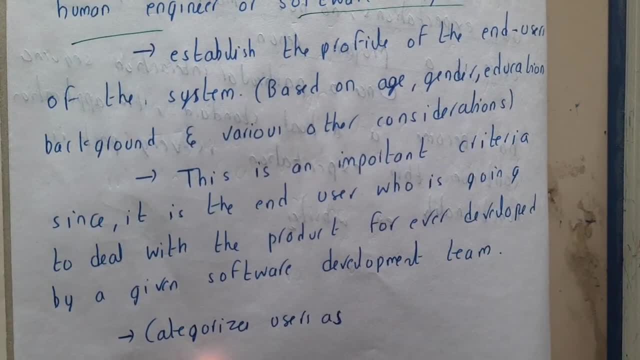 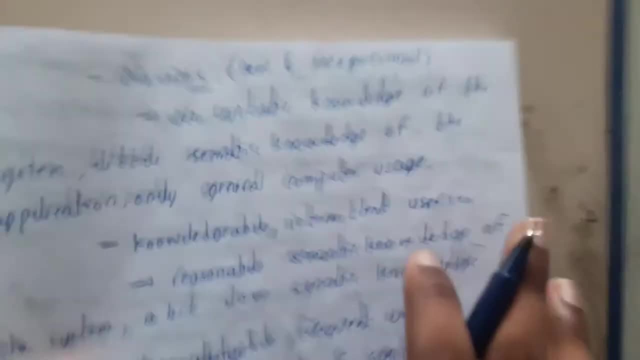 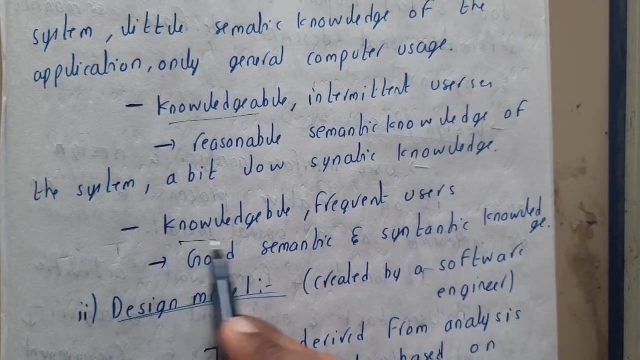 to deal with the product for after the development, right Forever after the development or after the deployment by the given software development team. These are categorized basically into two users: One is new and one is novices, and one is knowledged. and one is knowledged and frequently used guys. So infrequently and frequently used. 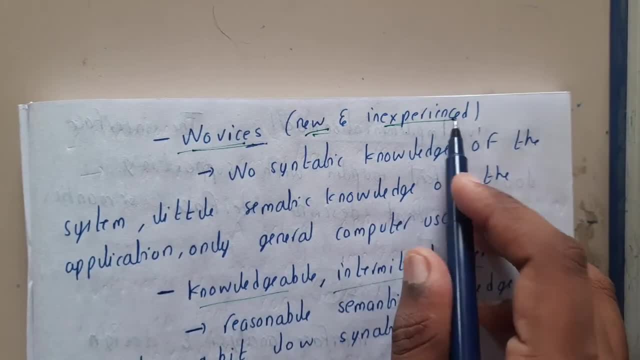 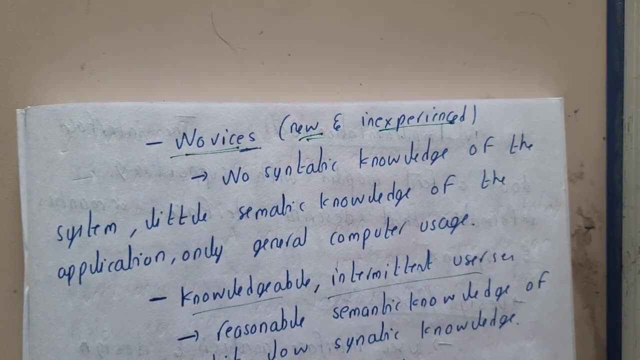 okay, So novices are nothing but new and inexperienced, So these guys do not have some technical knowledges and everything. guys, So they are new here and they are having no experience with any kind of previous apps like this or your application. okay, So no synthetic knowledge of 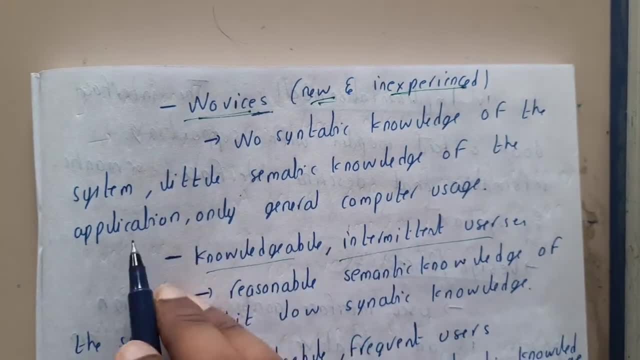 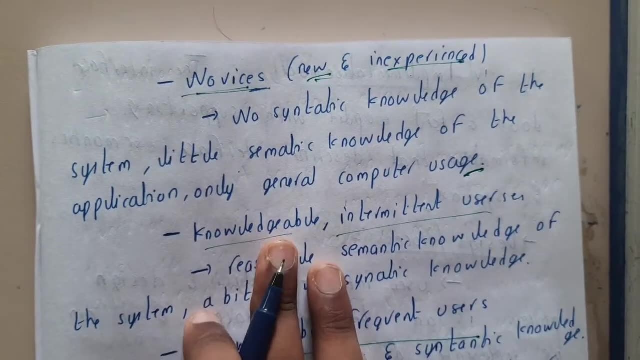 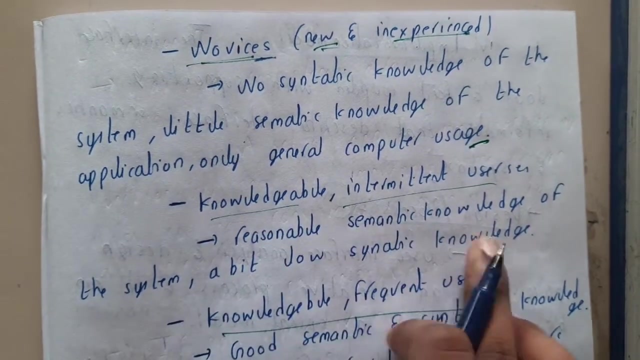 of the system. Little semantic knowledge of the application, only general computer users. So computer users will be known for them, okay, So knowledgeable. Knowledgeable are nothing but intermediate users. So these are also having some knowledge. So reasonable semantic knowledge of the system. 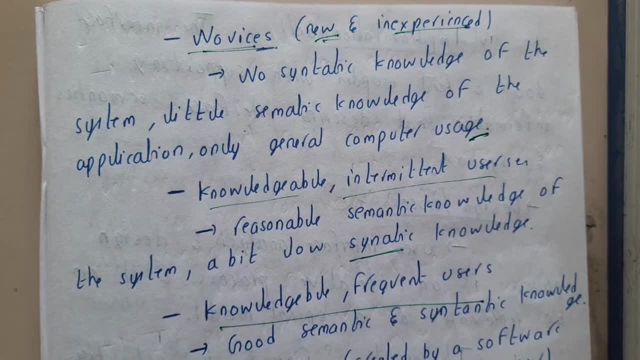 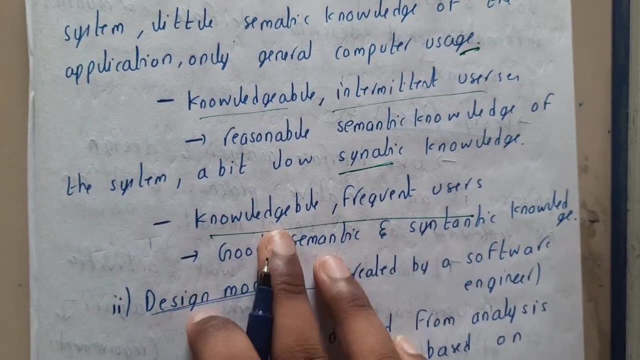 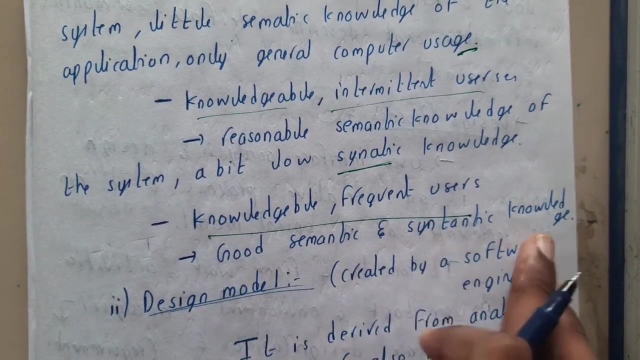 and a bit of low synthetical knowledge. So basically these guys also don't know that much about the coding and everything. So there are some other users who are called as frequent users and knowledgeable. So these are the common users which most of the applications will be having, So good semantics and synthetic knowledge. So basically,